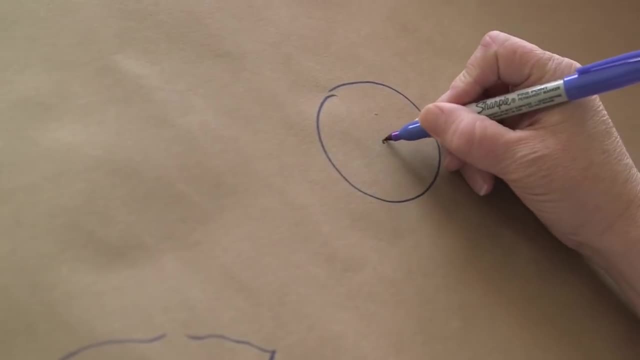 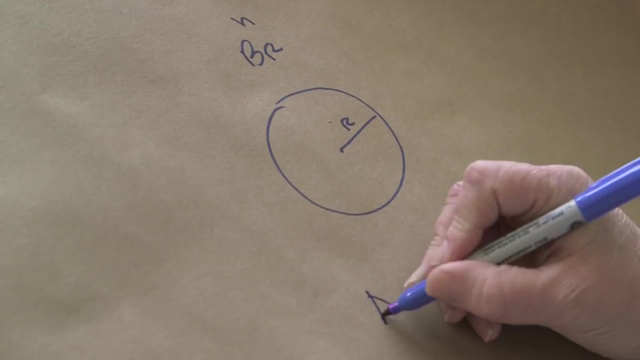 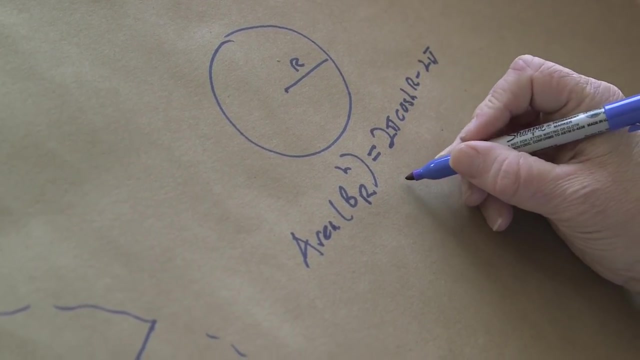 So one of them, if I draw sort of here, I'm in hyperbolic space and I have a ball of radius r, a ball of radius r in hyperbolic space. what is its area? So this is 2 pi cosh r minus 2 pi. Most people aren't familiar with that, but that's roughly pi times e to the r. 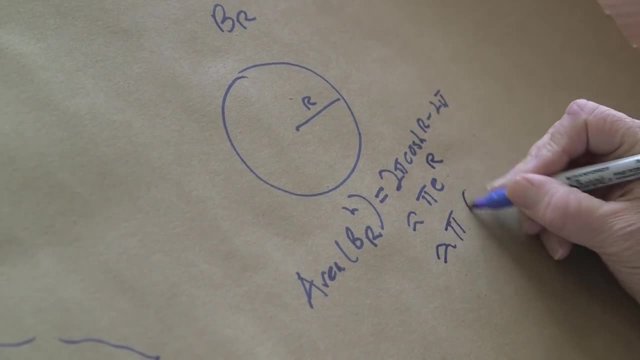 Now e is a number which is roughly 2 pi cosh r minus 2 pi. Now e is a number which is roughly 2 pi cosh r minus 2 pi. Now e is a number which is roughly 2 pi cosh r minus 2 pi. 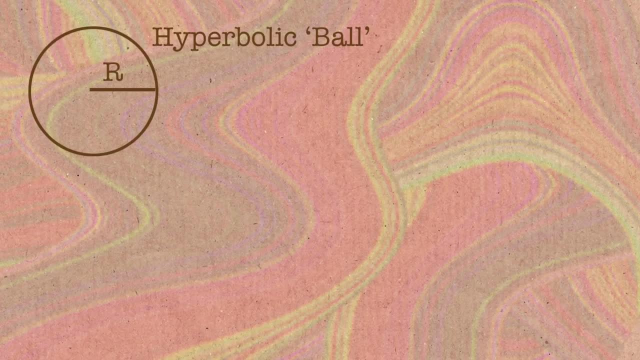 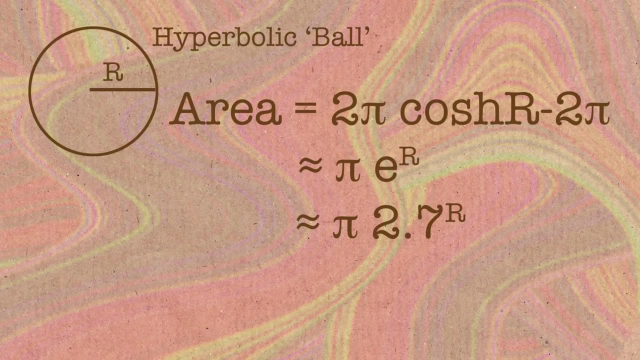 So that's roughly 2.7 to the r. So that means every time you increase your radius by 1, you multiply your area by about 2.7.. So we all know that if you start doubling, and you double over and over, you grow faster and faster. 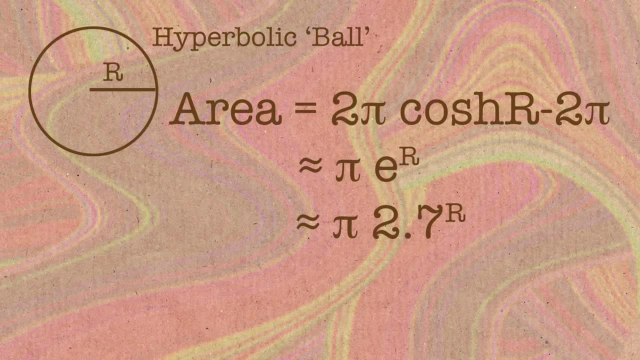 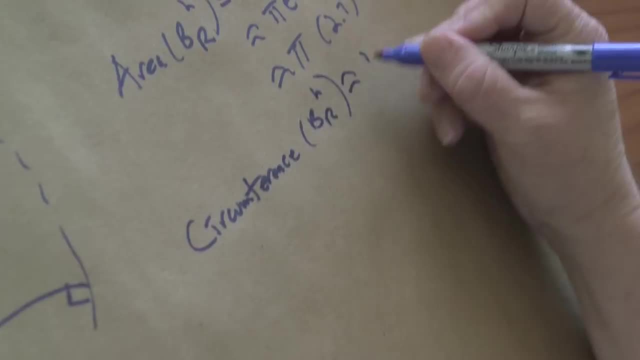 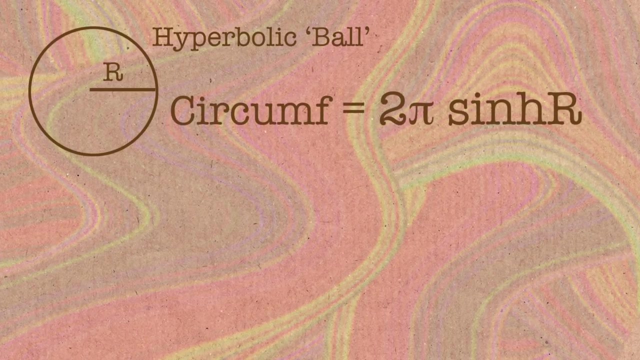 This is how compound interest works, And if you look at the circumference, or what's the length of the circle- some mathematicians would call it circumference- that turns out to be equal to 2 pi hyperbolic sine times r, And again that's roughly pi e to the r. 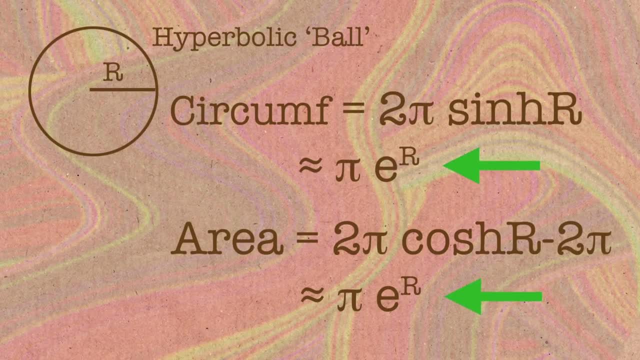 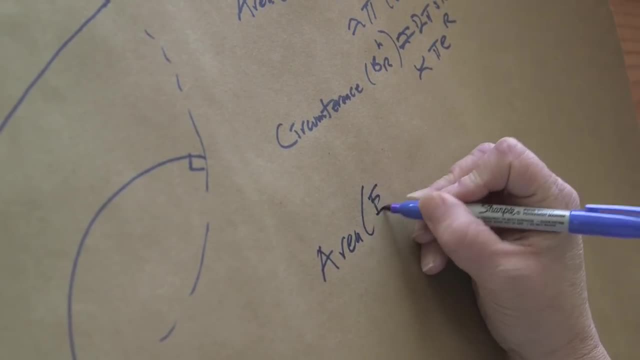 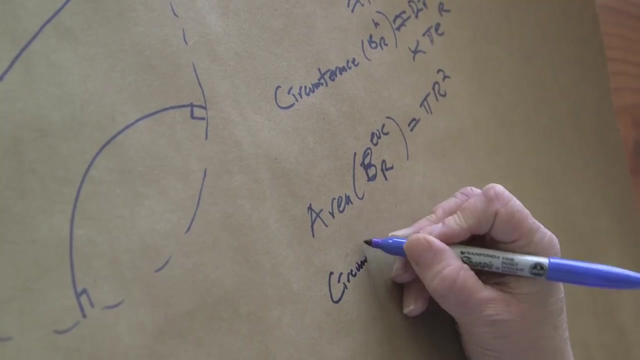 So the length of the boundary grows just as fast as the area does. Now let's compare that to Euclidean space. So remember, the area of Euclidean ball of radius r was pi r squared, and the circumference in Euclidean space, or the length of the circle in Euclidean space, is 2 pi r. 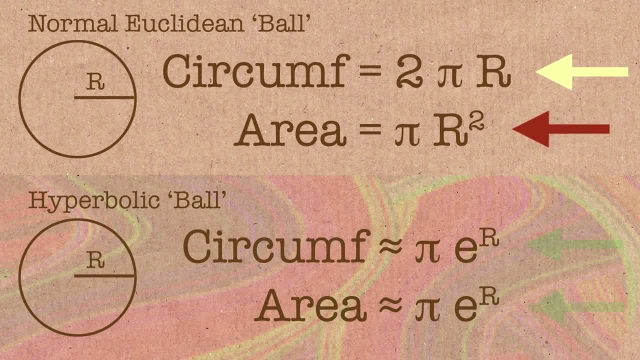 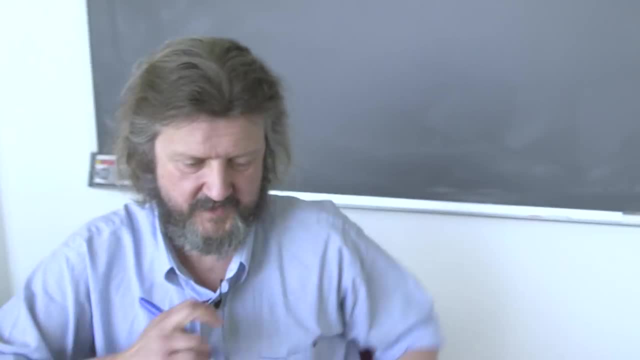 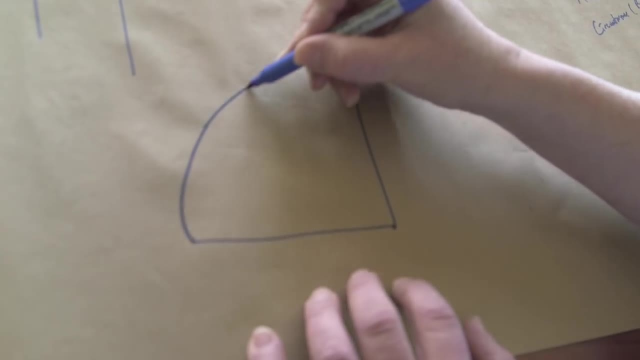 So this grows quadratically, this grows linear, and here both area and circumference grow exponentially at the same rate. Okay, let's think about what happens in baseball. So in baseball, we'll idealize this a little bit. So we're going to have a field. it's made up of a quadrant. 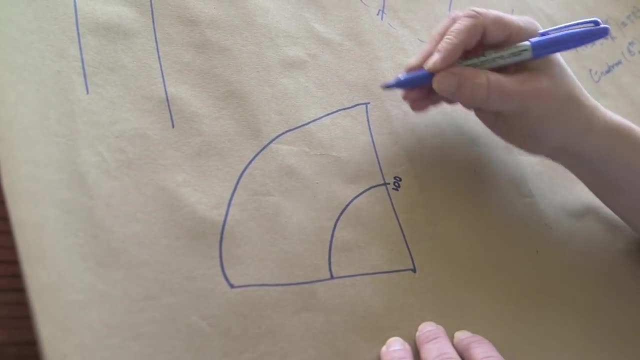 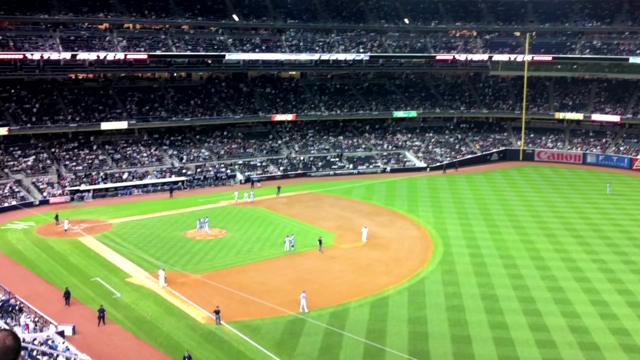 and the infield has radius 100, and the outfield has radius 300.. And so if you look at this guy, the area of this outfield is just over 60, is just over 60. If I remember right, it's about 63,000. 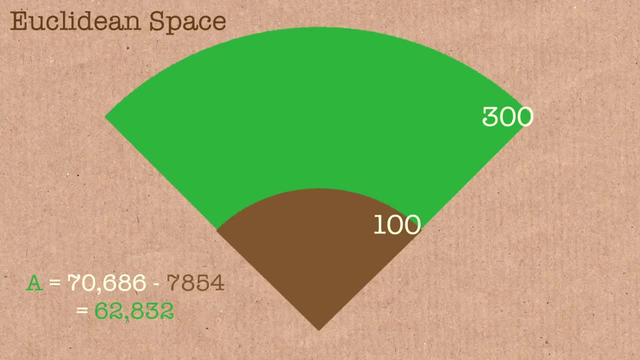 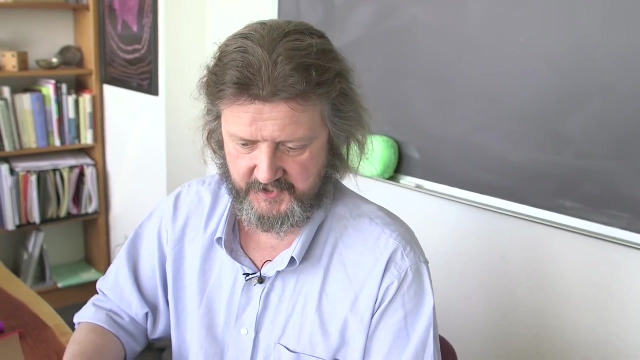 Okay, And so in American baseball we have three outfielders out here and they are able to cover most of the outfield, And so we can imagine that an outfielder can cover about 20,000 square feet. Well, what would happen in hyperbolic baseball if you took the same picture? 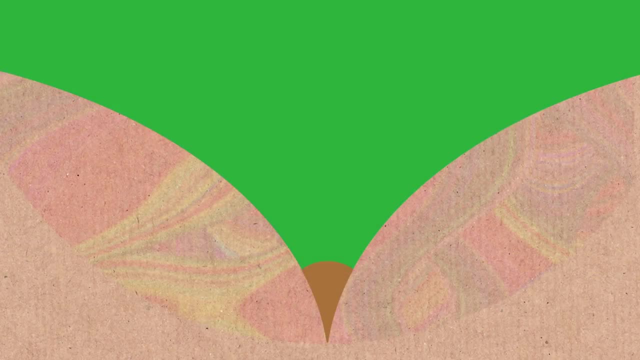 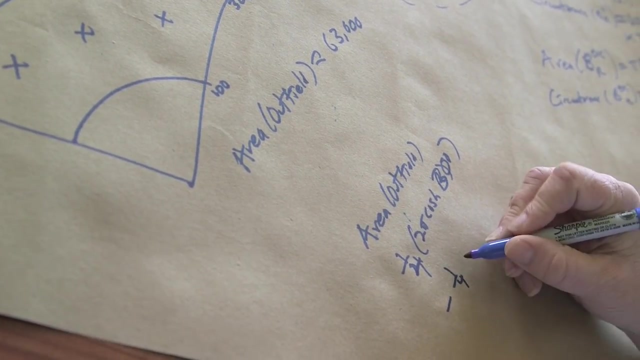 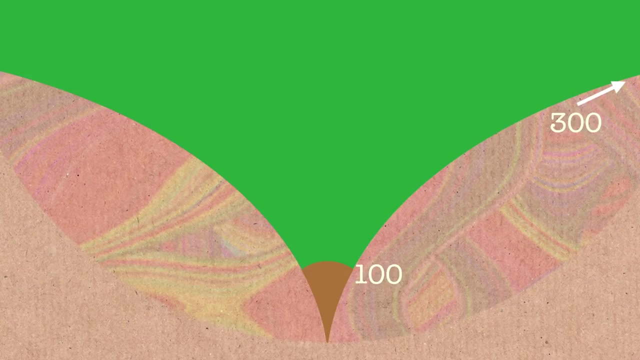 Well now the area of the outfield would be its 1 quarter, the area of the ball of radius 300, minus 1 quarter of the area of the ball of radius 100, and that's much bigger than 10 to the 99.. 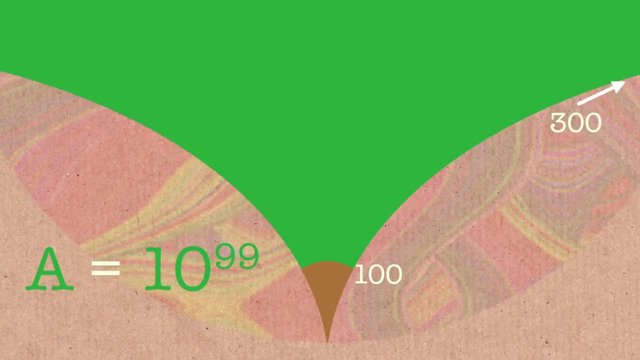 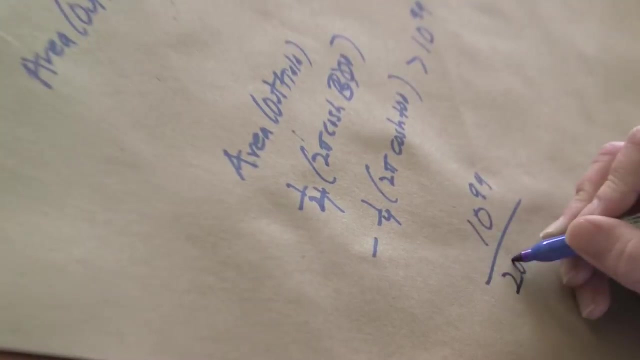 It's ginormous. So how many outfielders do we need? Well, if each of them can cover 20,000 square feet, which is sort of a dubious assumption, you need more than 10 to the 99 over 20,000 outfielders. 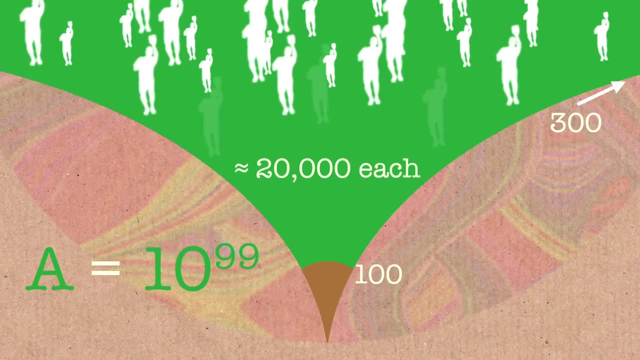 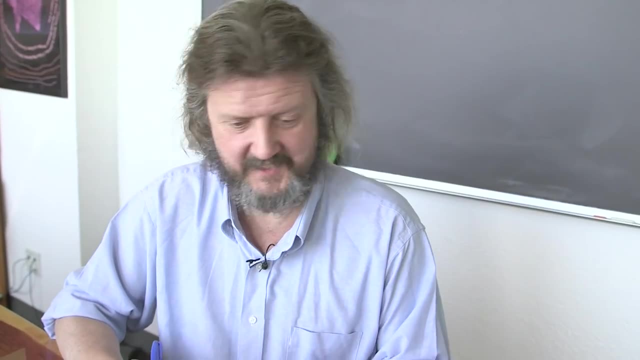 which is bigger than 10 to the 94. So one thing you can see here is you're not going to make any Disney movies about having a family big enough to have an entire baseball team. That's not going to work. Let me move to the next sport. 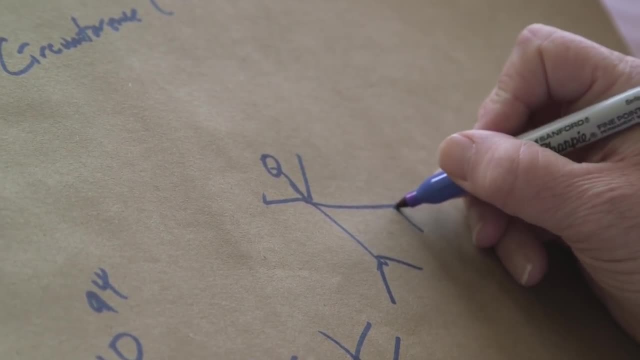 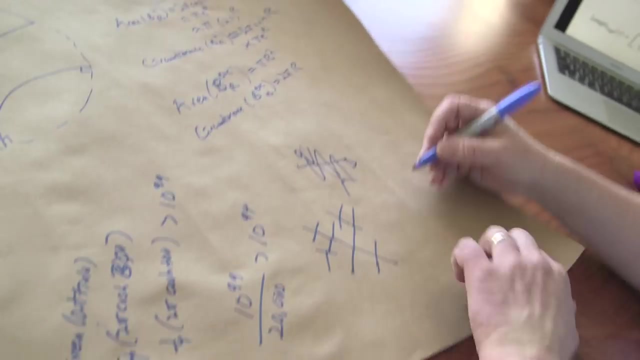 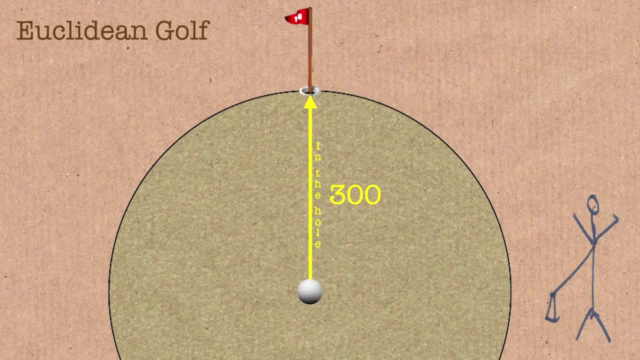 We'll talk about golf. So imagine you're a golfer here. Stick to mathematics, Professor, Anyway. so suppose you're standing here and your flag is over here, 300 feet away, You have a nice little wedge in to the hole. 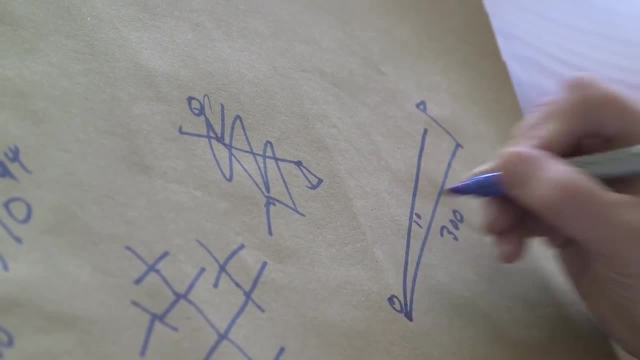 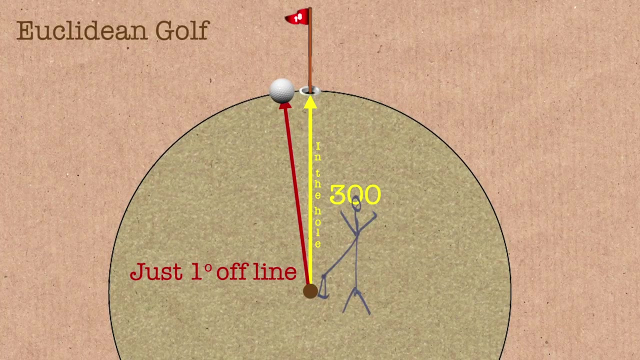 and you hit a very good shot. It's 1 degree off, But it's exactly 300 feet. How would you estimate that in Euclidean space You'd say: well, that's going to be roughly 1 degree's worth of a circle of radius 300.. 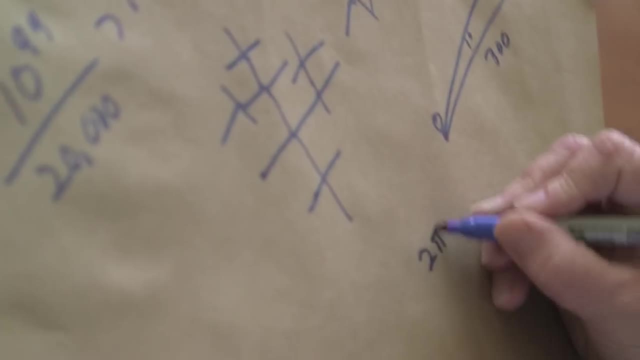 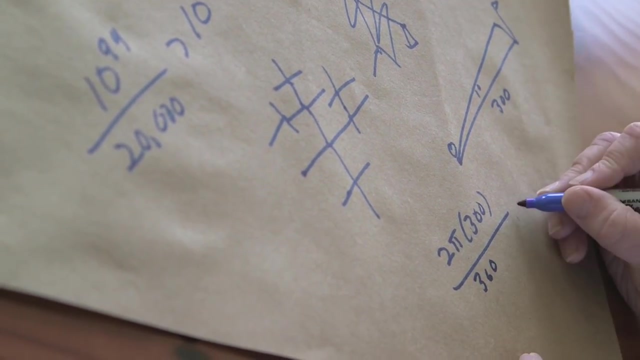 The circle of radius 300 has length 2 pi times 300, and then you take 1 degree worth of that, That's 1 360th. That turns out to be, if I remember right, something like about 5.23.. 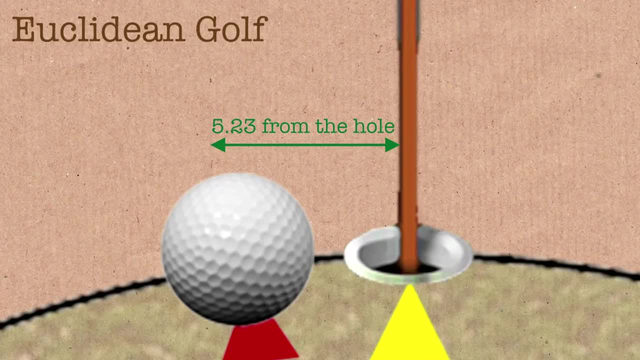 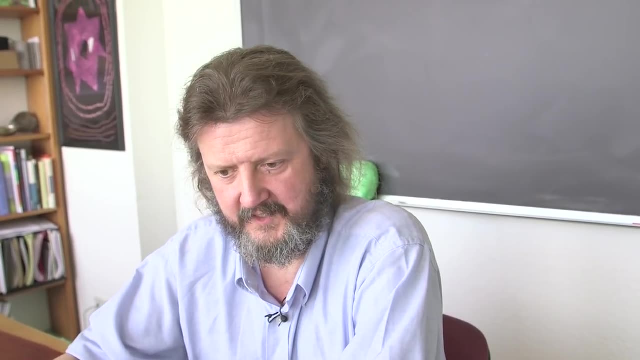 So you're about 5.23 feet From the hole. That's pretty good. You should be able to put that in. Well, you should, but I don't always do so. Now, what would happen if you did the same thing in hyperbolic space? 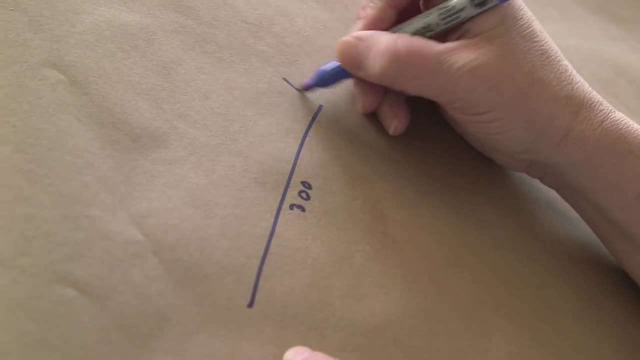 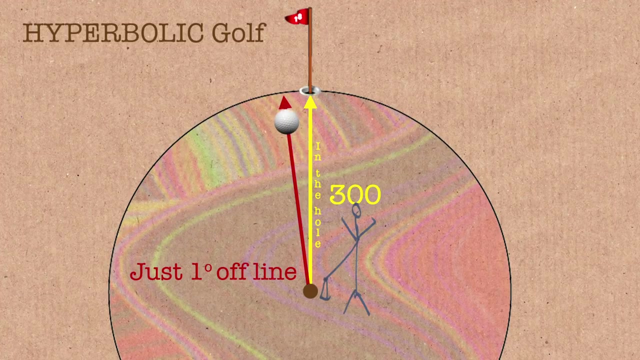 Now you're 300 feet. Here's your pin. You're 1 degree off. You hit it exactly 300 feet. You're feeling pretty good, So suppose we make that same estimate. Well, what's the size of a circumference of a circle of radius? 300?. 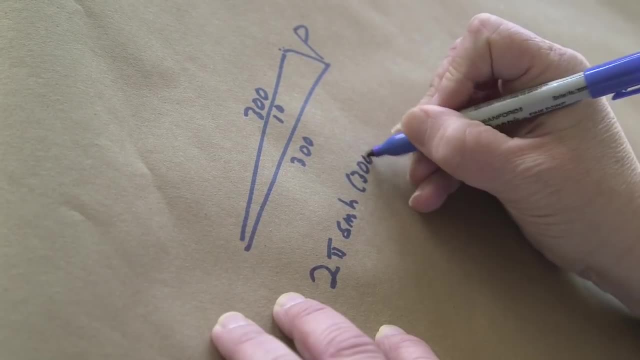 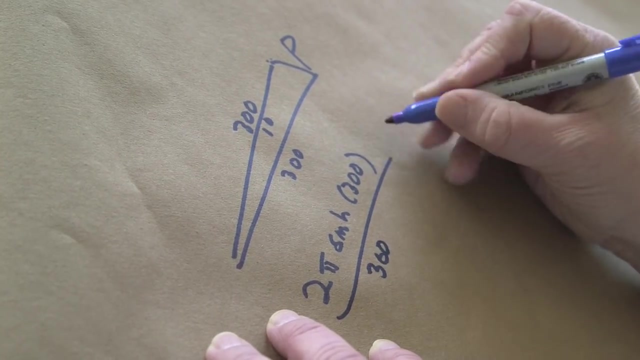 Well, that was 2 pi, since you have 300, which, remember, is like pi e to the 300. And now we're going to divide by 360.. Well, that's bigger than 10 to the 100.. 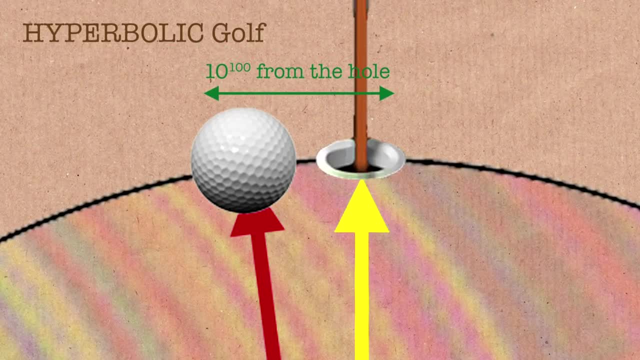 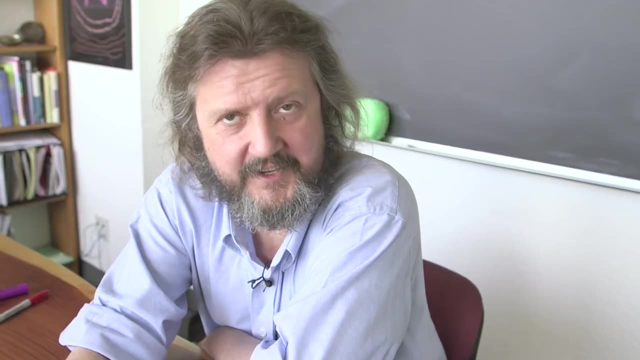 So this estimate suggests you're some number of feet which has over 100 digits away from the hole. Okay, so this can't be accurate because you know that you started 300 feet from the hole and you hit it 300 feet, so you're, at most, 600 feet from the hole. 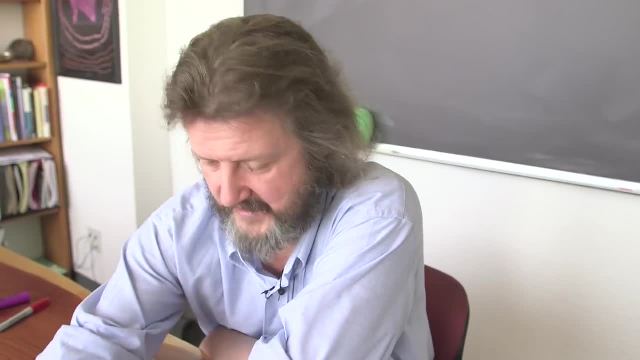 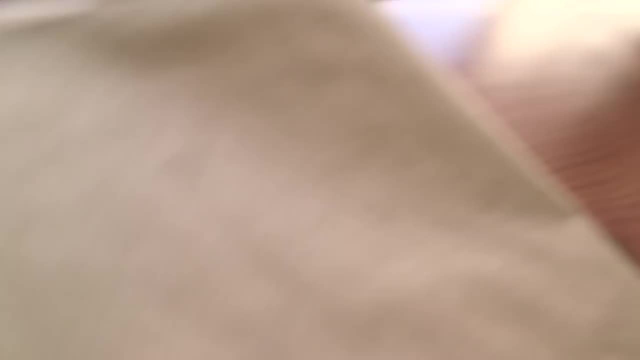 So we learned that this is not a very good thing to do and not providing a very good estimate. So, while it's in Euclidean space, walking around the circle isn't so very inefficient. In the hyperbolic space that's going to be a very inefficient way to get around. 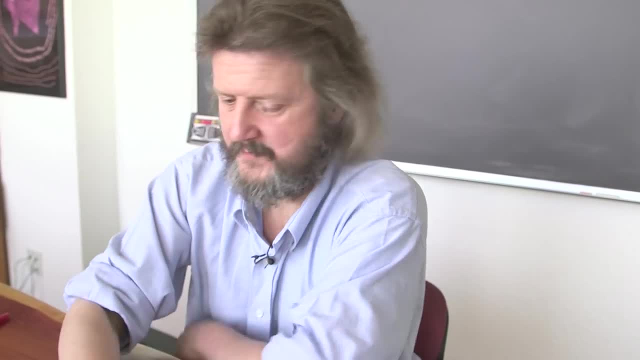 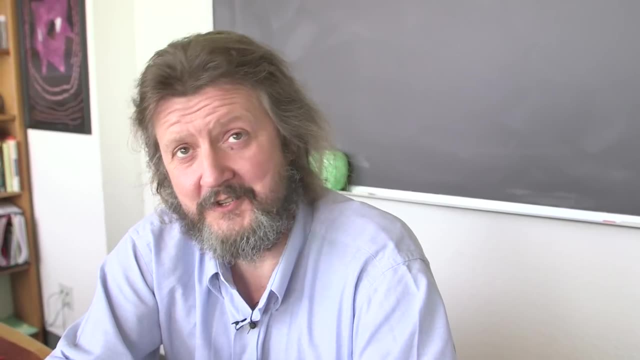 So how far are we from the pin then? So you can do a little bit of hyperbolic trigonometry and it turns out you're more than 590 feet from the pin, which is almost as bad as turning around and hitting it backwards. 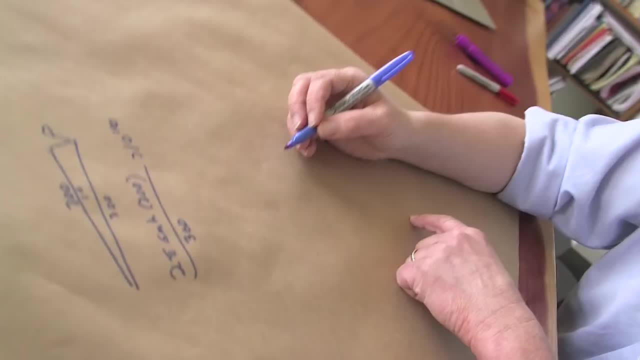 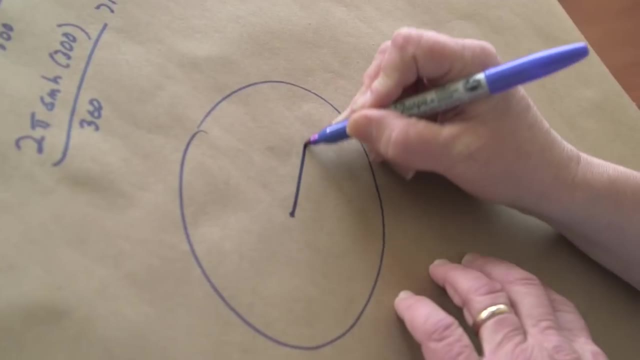 So hang on. what happened? Did it curve away or what did the ball do? One way of thinking about this is: what does this look like? Suppose you start at the origin, you travel 300 hyperbolic feet towards the boundary. 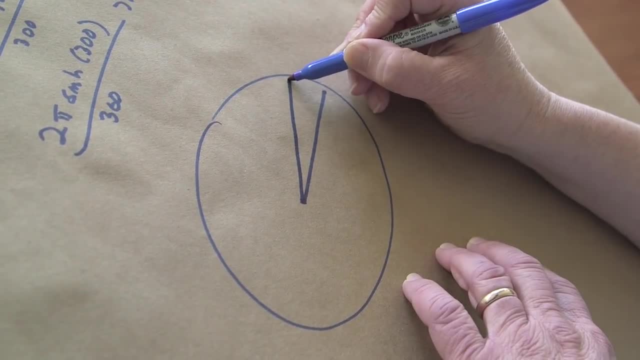 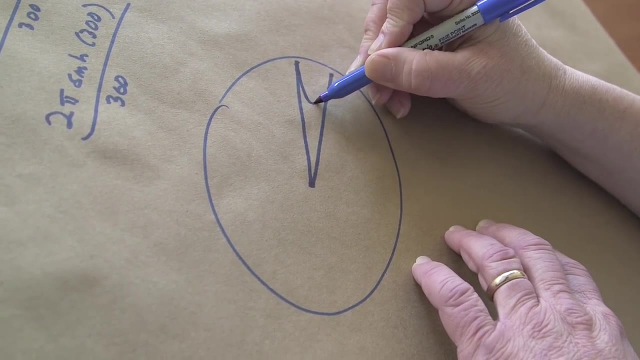 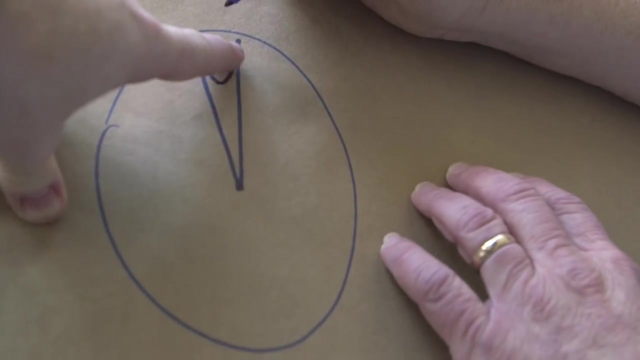 and then you're one degree off and you travel 300 hyperbolic feet towards the boundary. It turns out that the shortest way to get there goes all the way way back in and comes back out. Okay, so my second shot, my next shot, is going to have to follow a curve. that's so sharp. 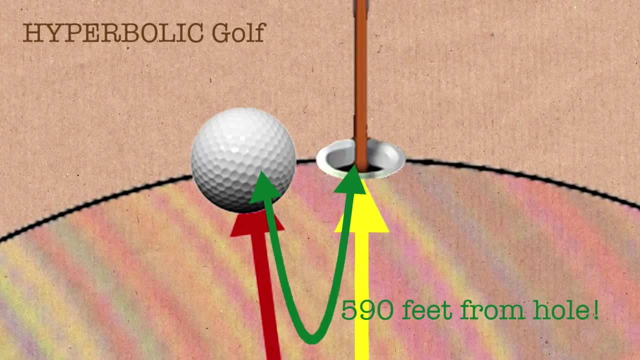 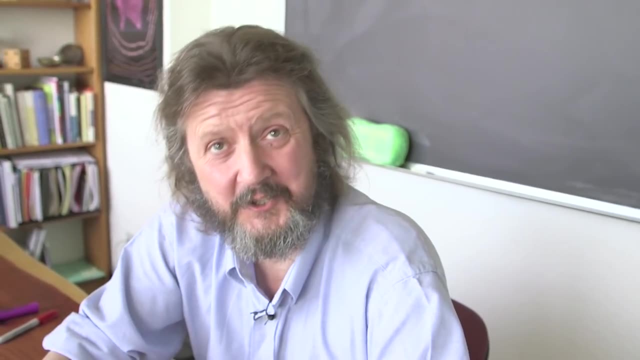 it's another big whack, Right. so you're likely- now you're 590 feet. now you're likely to be 1180 feet away after your next shot, even if it's very good, etc. So you're probably never going to get there. 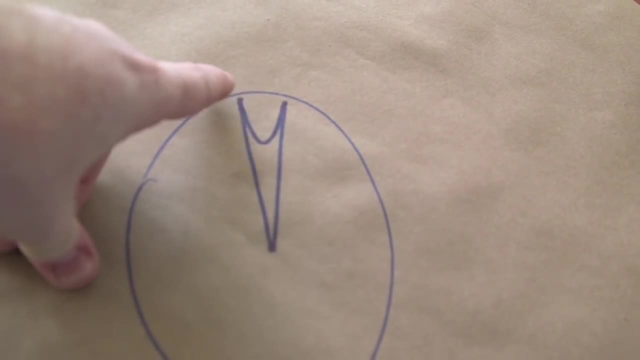 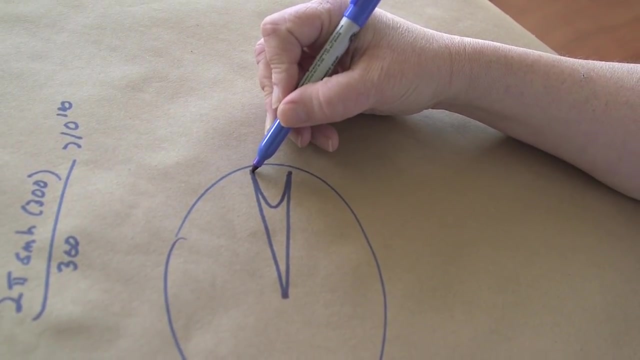 To my Euclidean eyes. I thought, oh wow, I'm really close to the pin now. this is easy, But in fact that path isn't open to me. or it is open to me Right? well, it is, but this turns out to be distance 10 to the 100.. 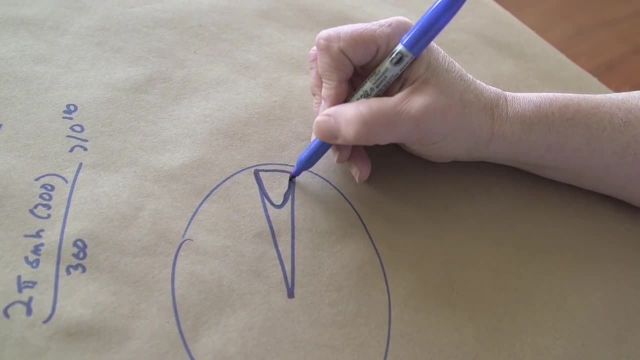 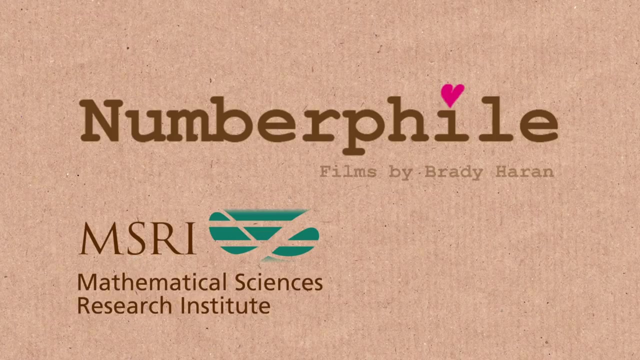 And if you want a path that is distance 590, it does something more like that. It goes back in towards the center and comes back out The outfielders. if you actually were, somehow they got the ball across the plate and you, despite not seeing it, until it was 6 feet from you.